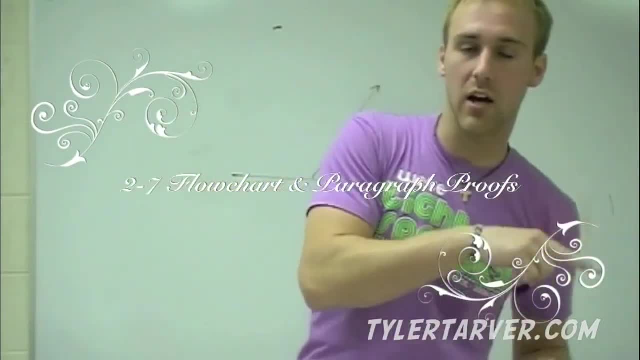 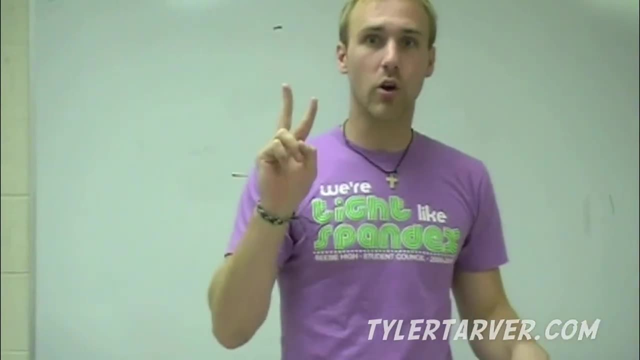 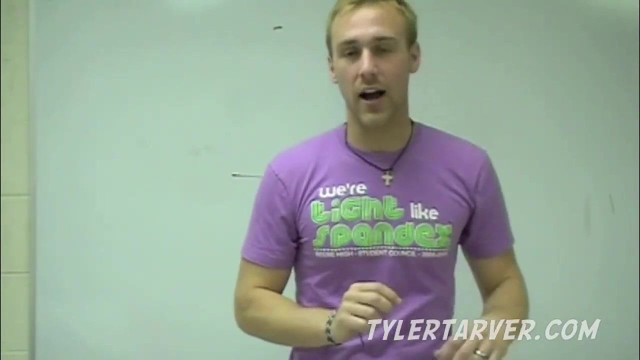 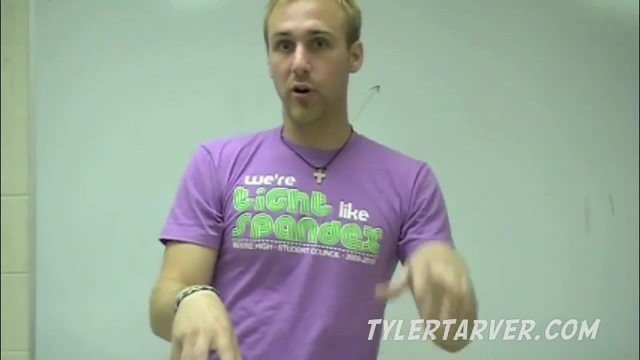 Okay. Last time, in section 2-5,, two times ago, I showed you an example of a two-column proof. They call it a two-column proof because math people are not creative. It's got two columns. It's a proof, You're done. Okay, It's like Bob's house- Guess whose house it is? Bob's, All right. Two-column proof means two columns. One is what you're doing, You're working the problem. The other is all the theorems and proofs that make you able to do that. Okay, Now, what we're learning today are flow chart and paragraph proofs. 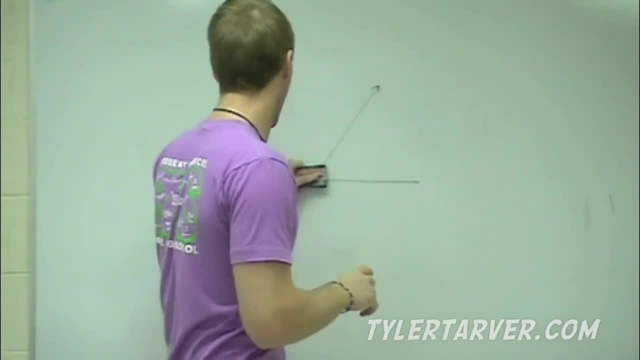 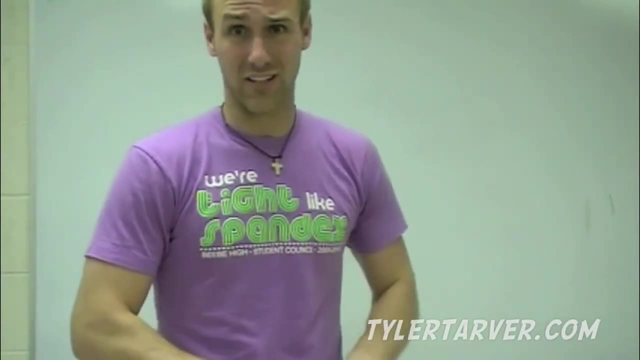 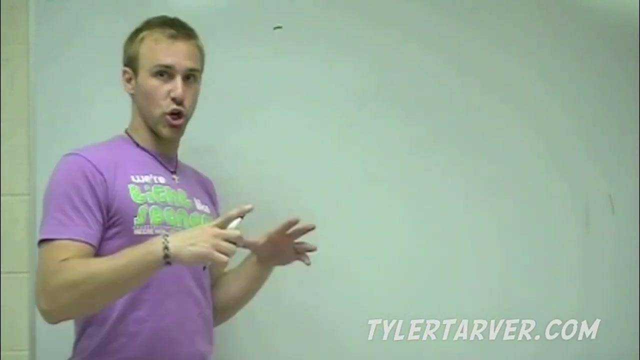 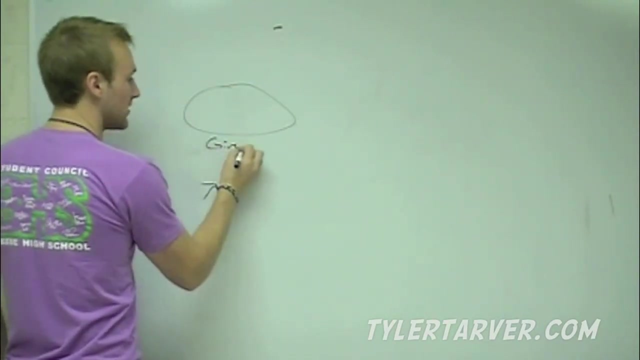 And paragraph proofs. I'm just going to run through this quickly. If you need to look through your book, you can do that. If you need to do more research, you need to ask whoever your real teacher is. Unless it's me, then just ask me. Okay, First we'll talk about: is a flow chart proof? Just like a sound. it's a chart that flows from side to side. All right, Usually you start with the you got the given. You write. It's just like in a two-column proof. You have the what you're doing and then you have the reasons statement and the proof. 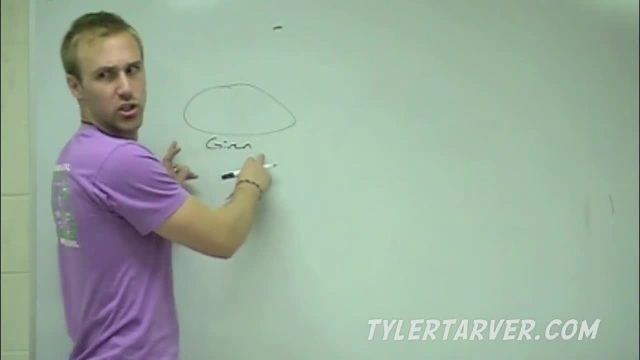 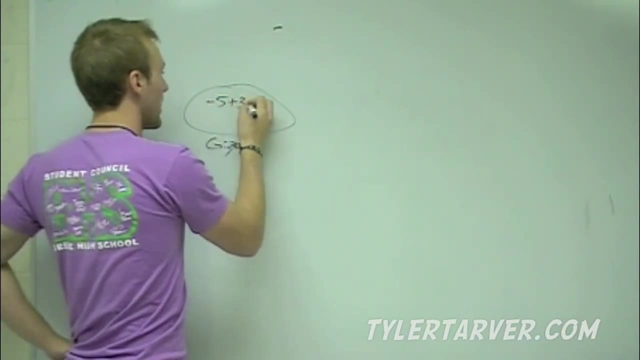 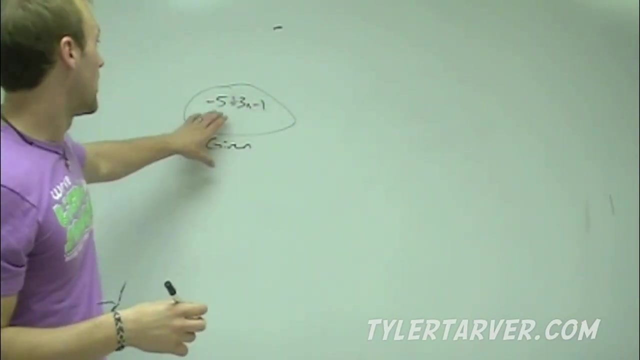 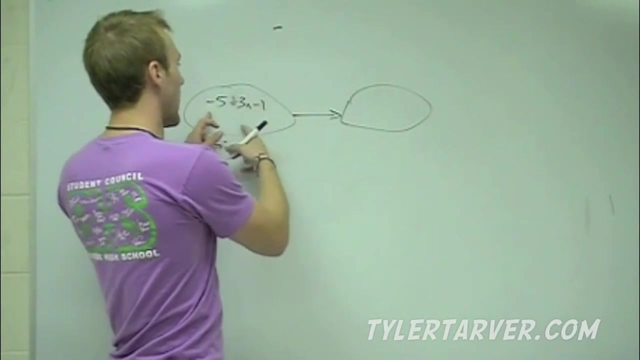 The reasons go right here, Statements go right here. So if it was like negative five plus three- and I'm sorry, negative five equals three and minus one, like it was that couple sections ago, that's the given, And then you just flow like this: All right, And then you would, you know, you would subtract, you would add one to each side. So we add one to each side. This would be the addition property. 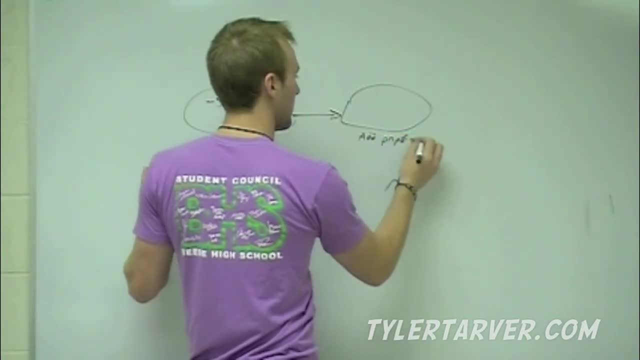 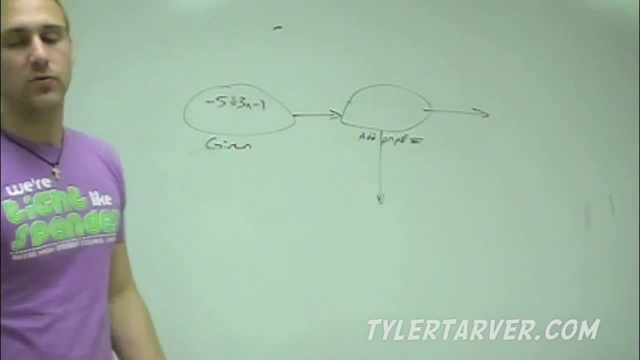 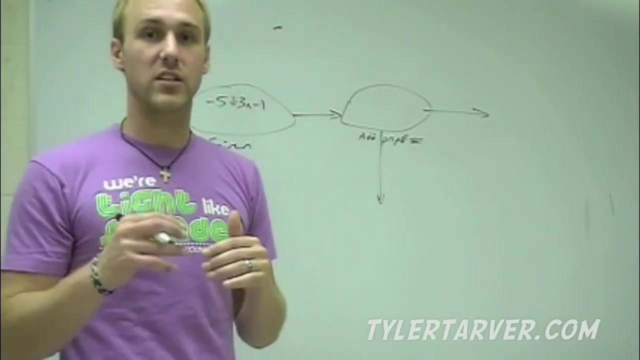 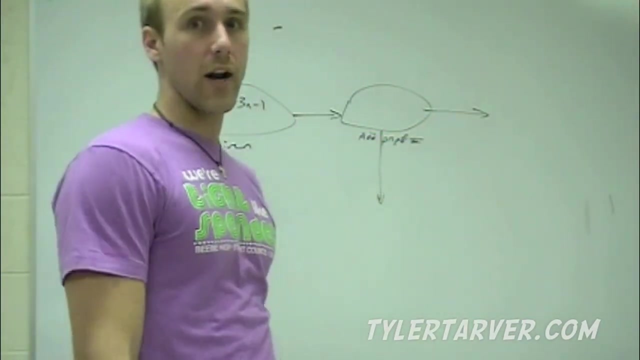 Of equality. You just put the, you just put that underneath there and then you keep going, Like if you have to split off in two different directions. I know this is very vague. I'm sorry. You don't use flow chart proofs that much, but you need to know them, So I'm giving you the basics, Okay. So what you're essentially doing is just like, if you know how to do a two-column proof, you can do this, Because all you're doing is you're putting the reason under here statement in the circle and then you're moving it with arrows until you figure it out. Okay, Sometimes they'll give you two givens. Then you start here and here and you go across Okay, And they'll move it.